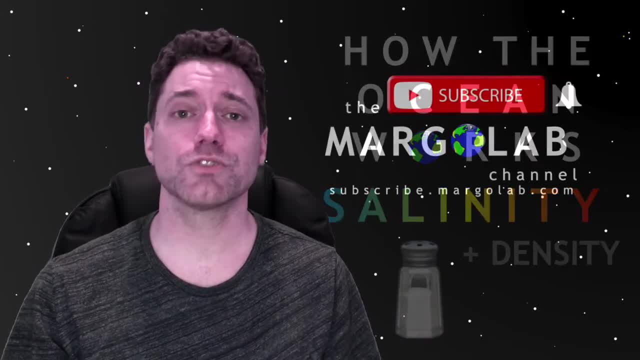 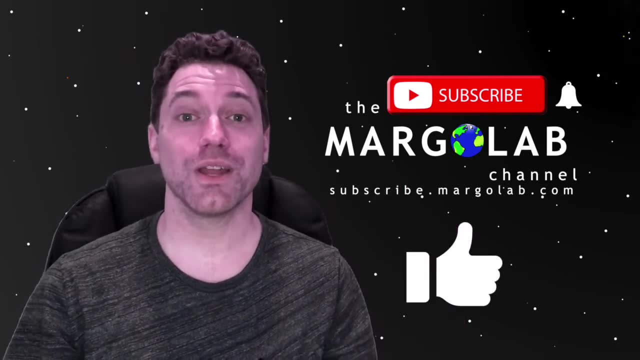 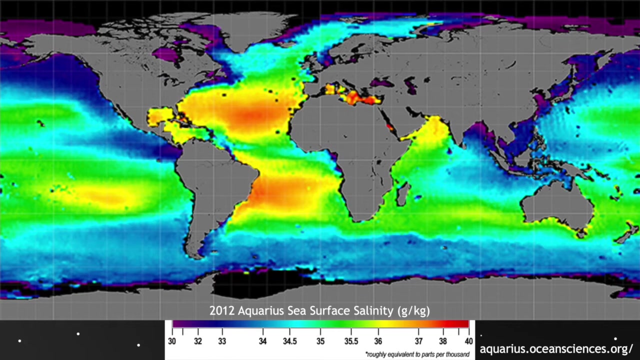 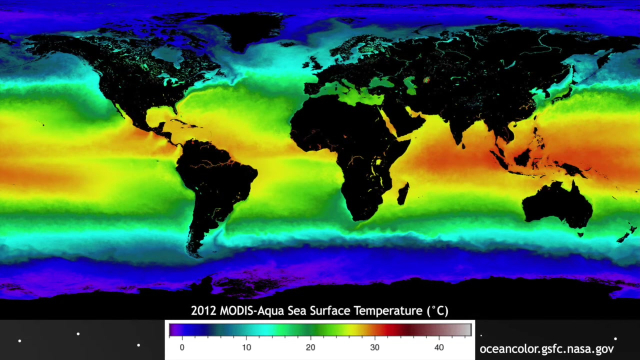 But before I get into that, if you enjoy this channel, make sure you support its growth by subscribing, and if you like this video, give it a thumbs up. All right, so now let's talk about salinity and the density of seawater. To start, here's a map of sea surface salinity measured by satellite, which is slightly more complicated than temperature, where the sea surface is warm near the equator and cold near the poles, as we'd expect. 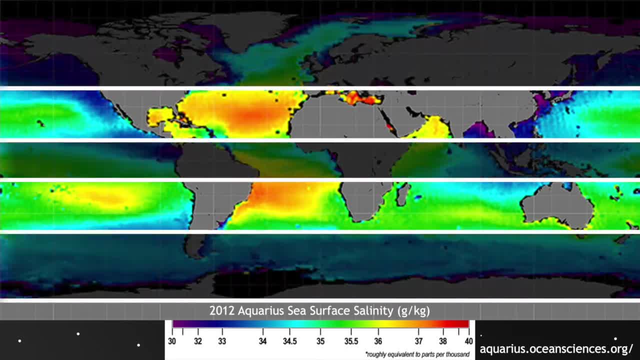 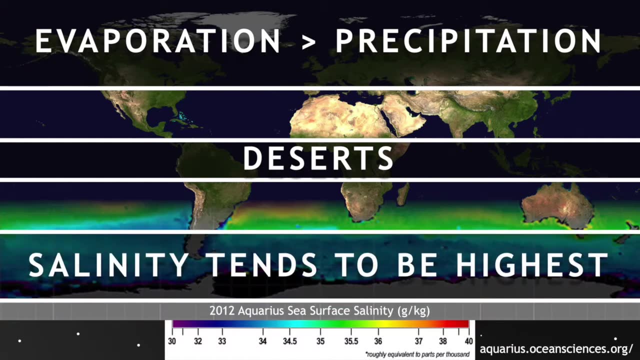 With salinity. it tends to be higher in areas where evaporation is greater than freshwater inputs, such as from precipitation and rivers, And, as you might expect, these latitudes correspond with deserts, which is where salinity tends to be highest. 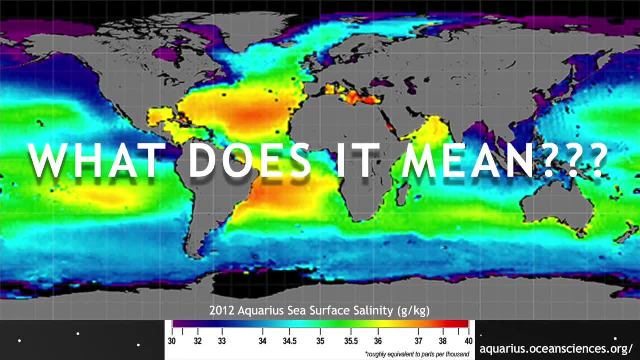 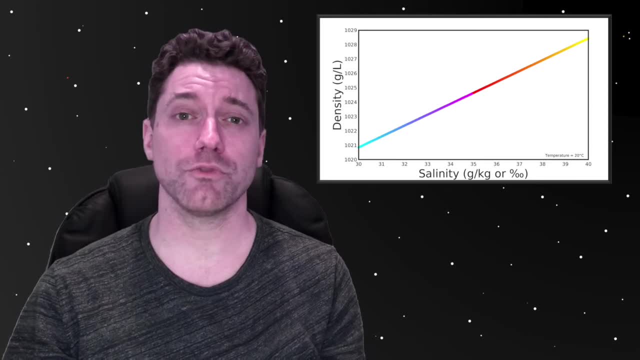 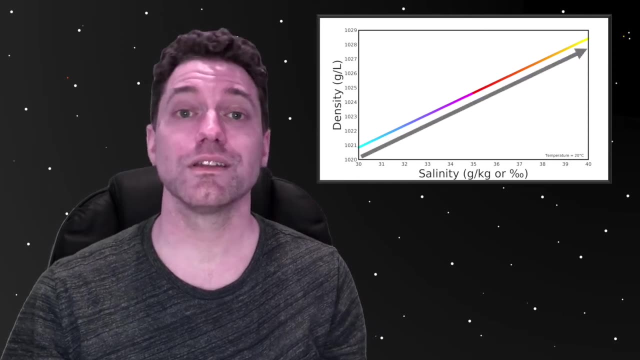 Now what does that mean in regards to density and water mass formation? Here is a graph that shows density in grams per liter or mass per volume, as a function of salinity. Generally, we can see that as salinity increases, density also increases. 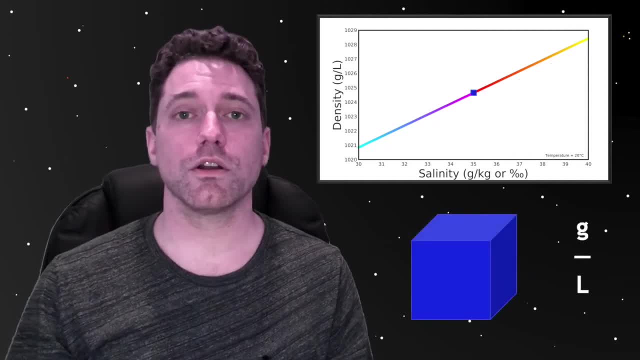 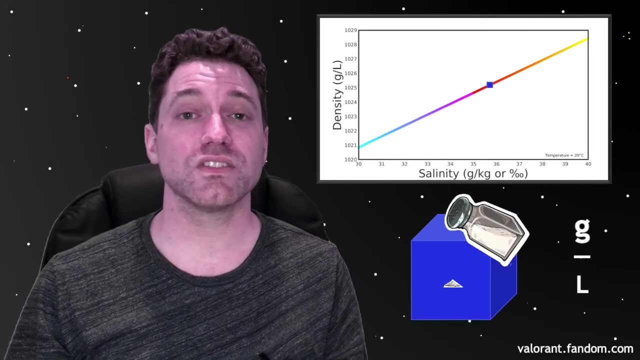 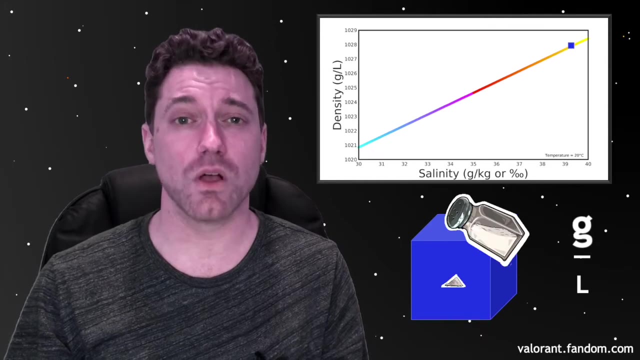 If we think about salinity as a function of density, we can see that density also increases, If we think about that conceptually, with this cube of blue water, as salinity increases, caused by more salt dissolving in the water, which does not change the size or volume of the cube but does increase its mass because it now contains more salt, which in turn causes an increase in density. 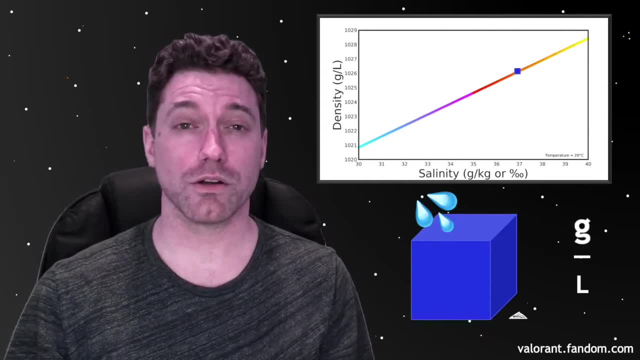 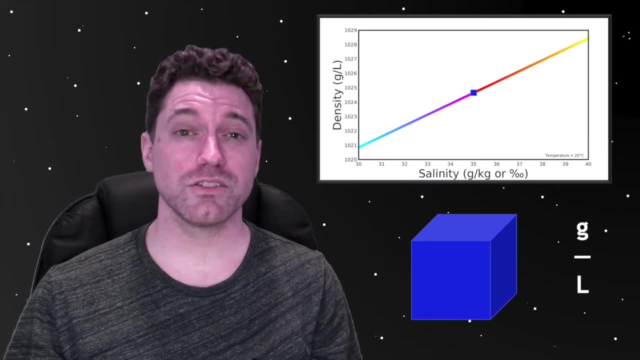 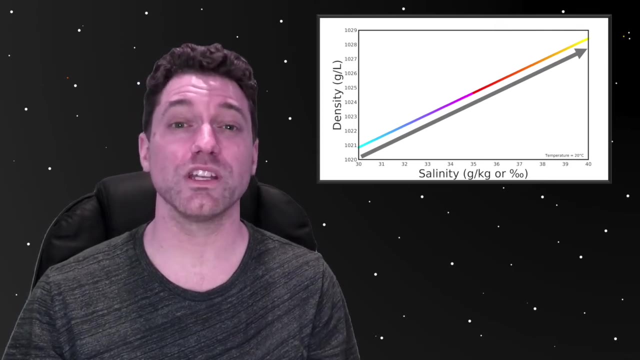 Conversely, if we decrease the amount of salt in the water, the mass of the cube will decrease, making it less dense. Considering what we've learned about the relationships between temperature and salinity with density, it makes sense that the densest ocean waters are going to be the coldest and the saltiest. 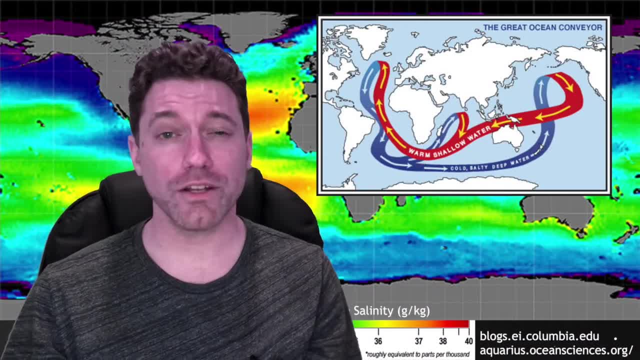 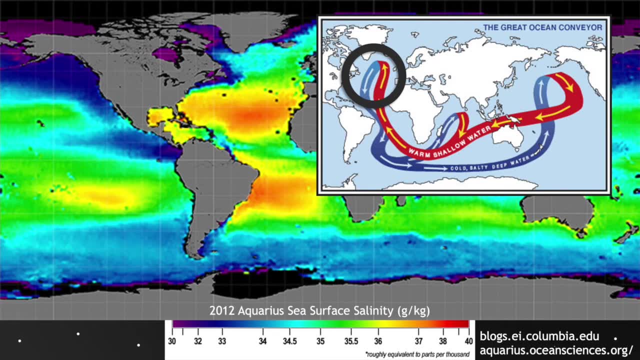 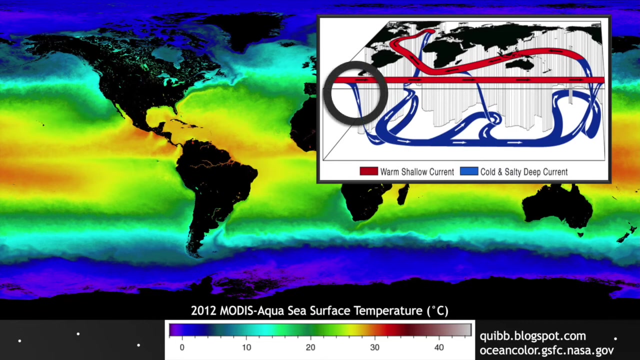 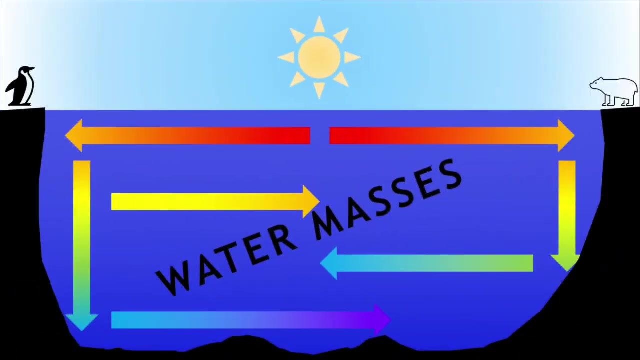 And now, if we look at this schematic of the Great Ocean conveyor, as well as salinity, our view and temperature, we can see that there is also deep, or rather bottom water formation around Antarctica. now, considering everything that we've learned in this schematic of water masses from last week's video, if we look,